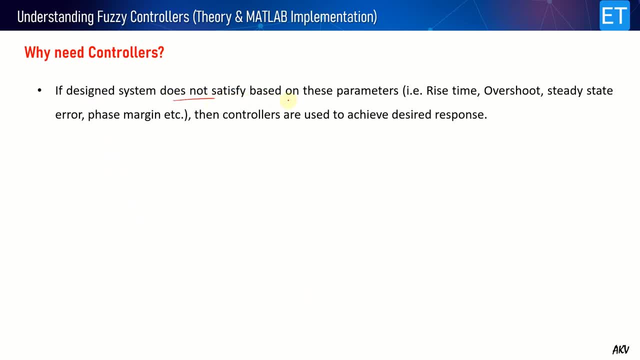 if design system does not satisfy based on the following parameters like rise, time overshoot, steady state, error or phase margin, etc. Then controllers are actually used to achieve the desired response. Controllers are actually the system response modifiers. A controller is mainly introduced. 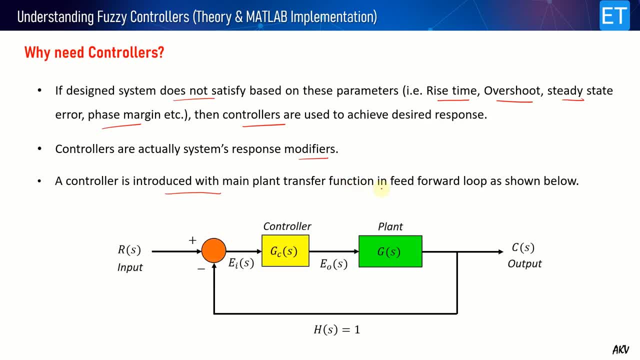 with the main plant transfer function in feed forward loop, as shown below. So this is a plant in a feedback system and this is the controller. So here controller is actually modifying overall system response by relocating the poles at the desired locations, by modifying the overall system transfer function. 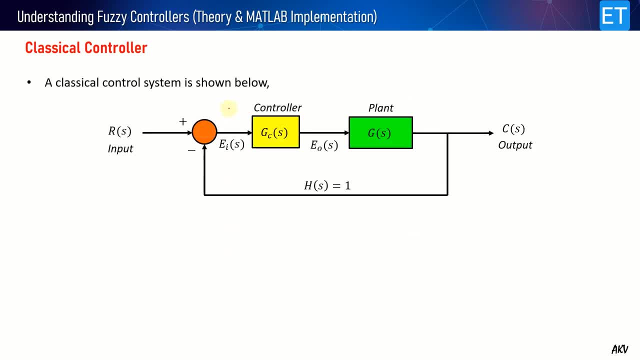 So now let's see the classical controller. Actually the placement of the classical controller is shown in this figure. In this system this controller actually works on the crisp input values and provides the crisp output values. So here controller has actually a precise mathematical model. So this mathematical 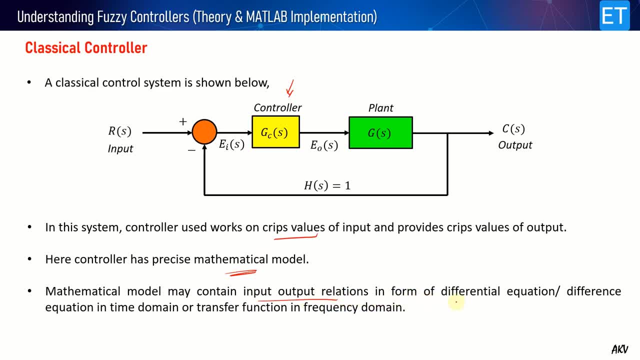 model may contain the input output relations in form of either differential equations or difference equations in time domain, And if you're talking about the frequency domain, you're talking about the frequency domain. So this mathematical relationship is in form of the transfer function as shown here, like GCS. 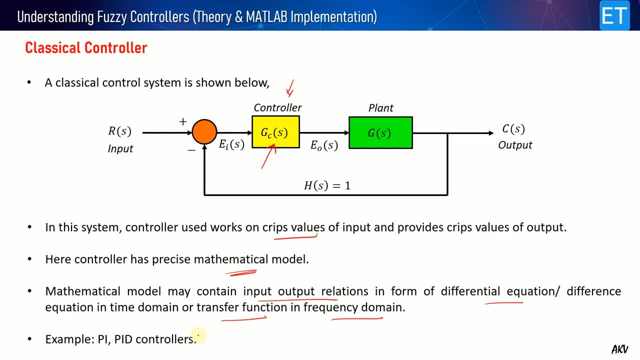 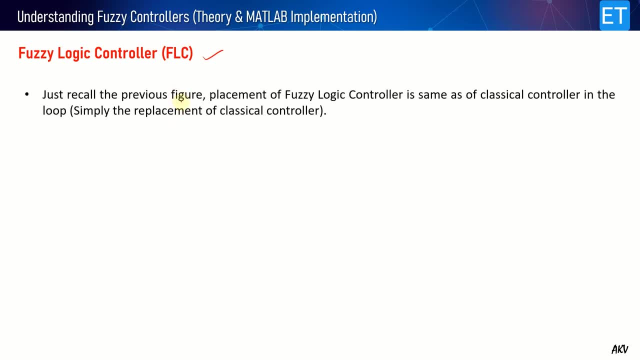 And examples are like PI, PID controllers. These are classical controllers. So now let's see what is a fuzzy logic controller actually? Just recall the previous figure: The placement of FLC is same as of the classical controller. I mean, connection wise, they both are same. 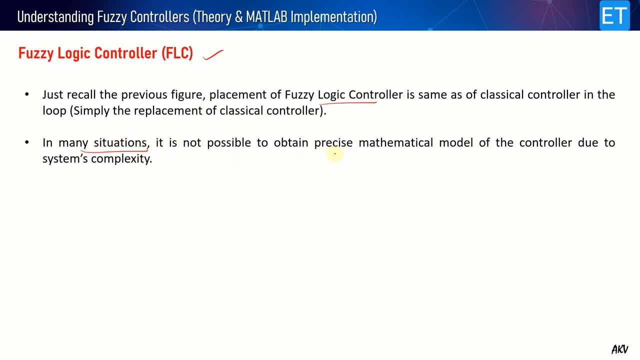 But in many situations it is not possible to obtain the precise mathematical model of a controller due to the system's complexity. So in such case of vague, ill-defined and the complex system model, the one impressive solution is the fuzzy logic based controllers. 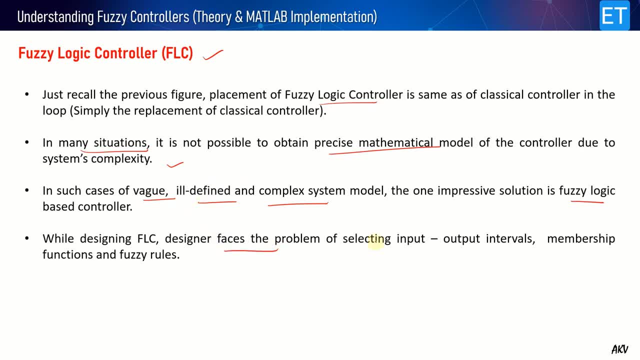 So while designing FLC, actually designer faces the problem of selecting input, output variables, Bamber shift functions and then fuzzy rules. So that is actually the main difficulty. So the success of the design actually depends on the designers experience. So in another approach, FLC can also be combined with these conventional- I mean the classical. 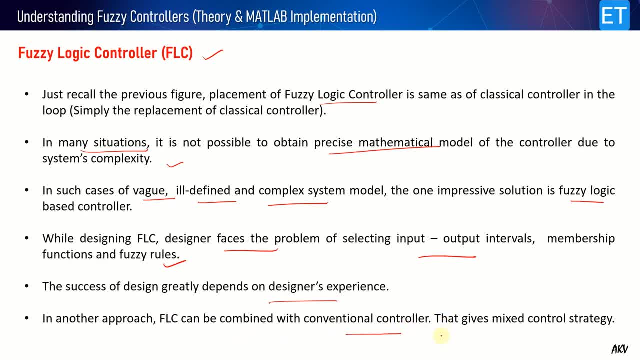 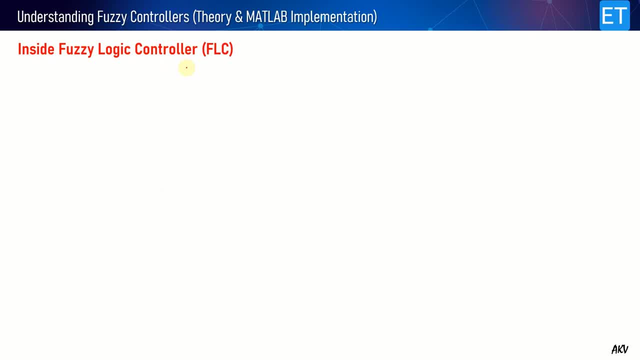 controllers. So that gives actually the mix control strategy. So in this video I'm just talking about the FLC only. So now let's see what is inside the fuzzy logic controller. It's basic architecture, I mean. So actually FLC works on the fuzzy values, not on the classical. So let's see what is. 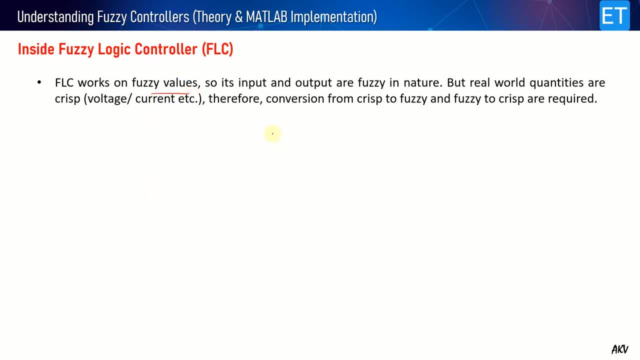 inside what is inside of FLC, So? so let's see what is inside of FLC. So what we can judge is that it controls the feedback value of the design, And then we can set some values, crisp values. so both the inputs and outputs are fuzzy in nature, so, but we know that real. 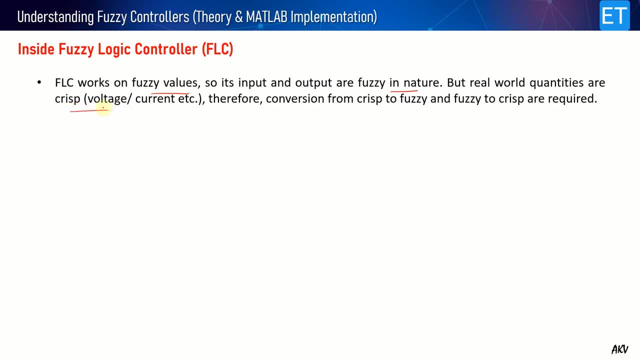 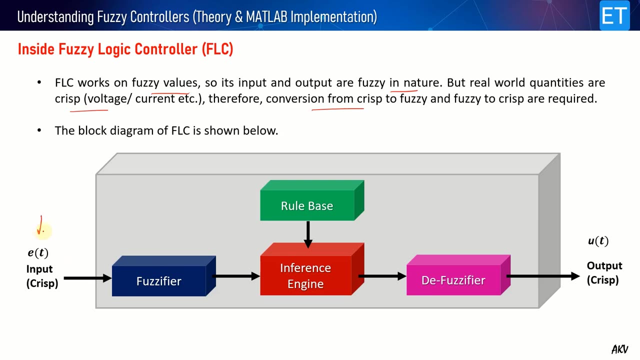 world. quantities are not fuzzy, they are crisp, such as some voltage or current in magnitude. therefore conversion from crisp to fuzzy and fuzzy to crisp are required for the FLC. So the block diagram is shown here. so this is your crisp input. so first you have the 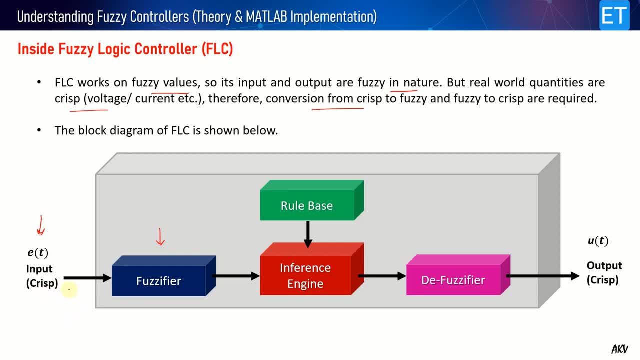 fuzzy fire which changes these crisp values to the fuzzy values, and similarly at the output stage we have the defuzzy fire which converts the fuzzy values into the crisp output values so that can be given to the plant. Here we have the rule base where all the rules are defined, and this is the inference engine. 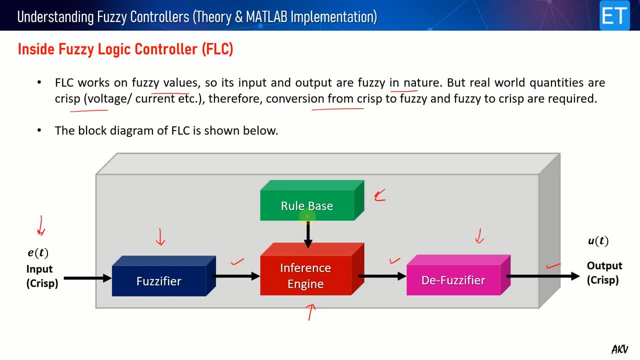 so, on the basis of the inputs, it activates certain rules and gives a fuzzy output. so all these fuzzy outputs are aggregated and then they are defuzzified to get a single crisp output. So FLC can be MIMO. I mean multiple input, multiple output systems. it can be designed, even the 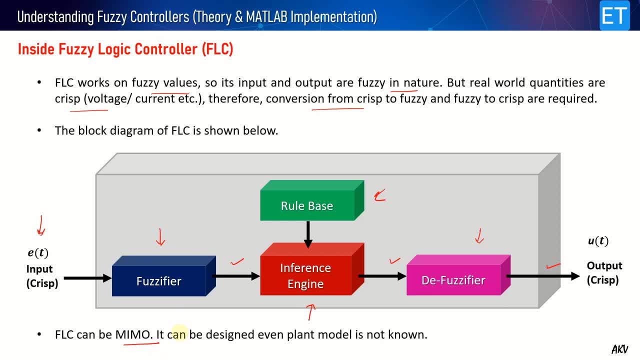 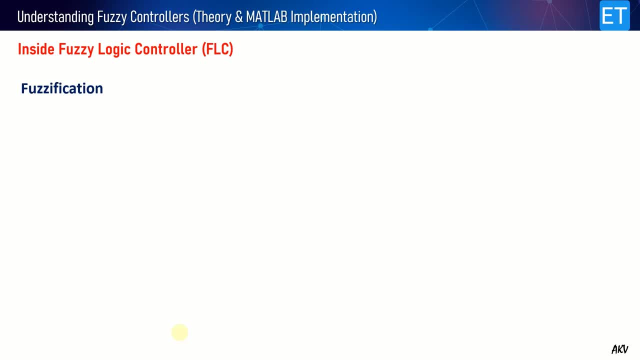 plant model is not known. even if you don't have any idea about the mathematical model of the plant, still you can design the FLC. So now let's see the it's basic steps. I mean what, how to do it. So let's see what happens inside the fuzzification. so fuzzification is a process of transforming. 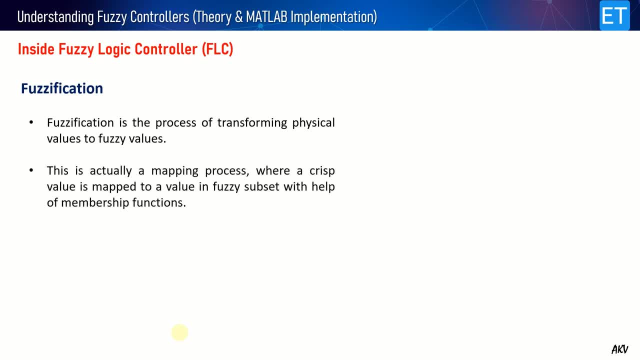 physical crisp values to the fuzzy values. so this is actually a mapping process where a crisp value is mapped into the fuzzy subset with the help of some membership functions. So these membership functions actually assign the degree of the membership in the range 0 to 1 to those crisp values. 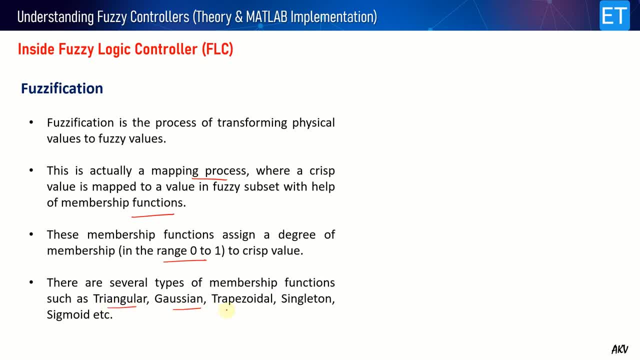 So there are several types of membership functions, such as triangular, Gaussian, trapezoidal, singleton, sigmoid, etc. Depending on the requirement, we choose the appropriate membership functions. So here in this example you can see that how the crisp values are fuzzified. 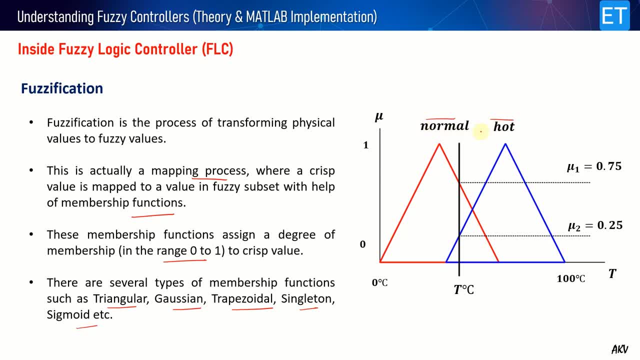 So we have the two fuzzy subsets, normal and hot, for the temperature T, and this is my input temperature, let's say some T degrees Celsius. that is a crisp value. So you can see that this crisp value is cutting this normal fuzzy value Fuzzy subset at this point and it is cutting the hot at this point. 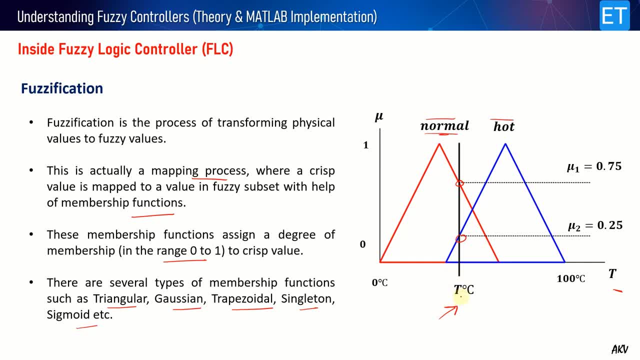 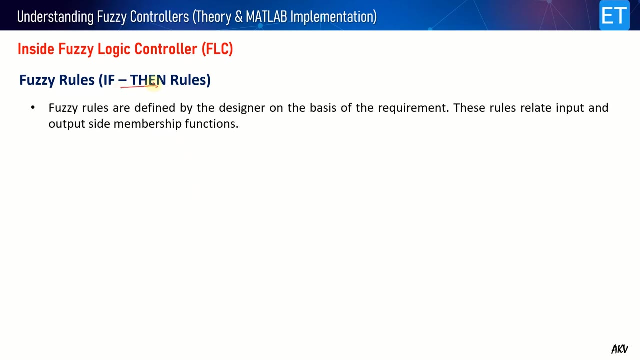 So I will say that this crisp value is 75% belonging to the normal set and 25% to the hot fuzzy subset. So this is how your crisp values can be fuzzified in the fuzzy logic. So now come to the fuzzy rules. they are also known as the if then rules. these fuzzy rules. 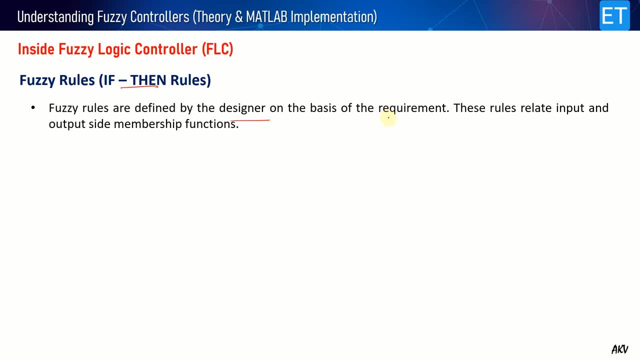 are actually defined By the designer on the basis of the requirement. it actually requires the experience. So these rules relate input and output side membership functions. So actually their structure is: if, then structure. For example, if your system has single input, then the rules structure will be like this: 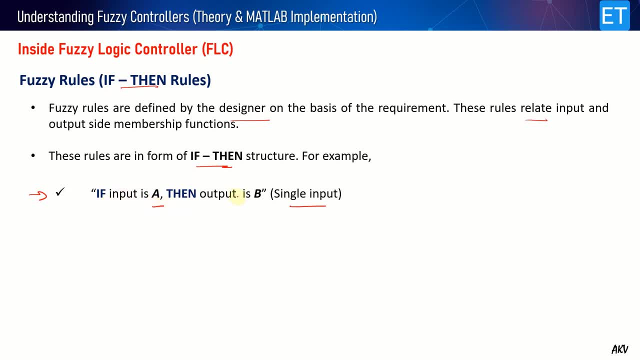 So, for example, if input is A, then output is B. If you have the multiple inputs, Let's say two inputs, then the structure will be like this: If service is excellent or food is delicious, then tip is more. So this is the case for multiple inputs. here we have used the two inputs, service and food. 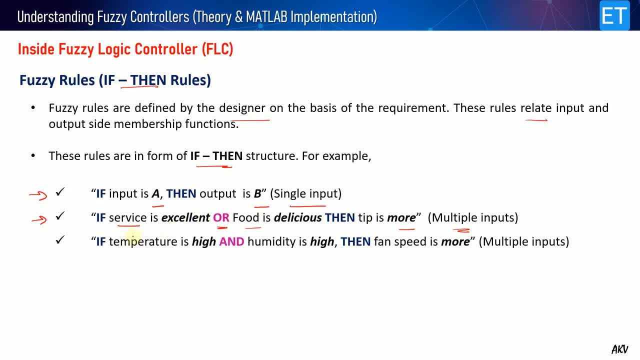 and the output is tip. Similarly- this is another statement- if temperature is high and humidity is high, then fan speed is more. So here the temperature And humidity are two inputs And the fan speed is the output. So what is the difference between these two rules? the here the difference is of this operations. 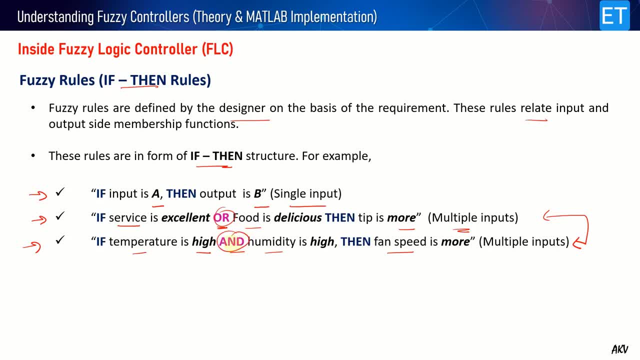 or an end operations. So these are few examples of fuzzy rules Here, if part is known as the antecedent and then part is known as the consequent. So here antecedent relates input side membership functions, while consequent relates output side membership function. 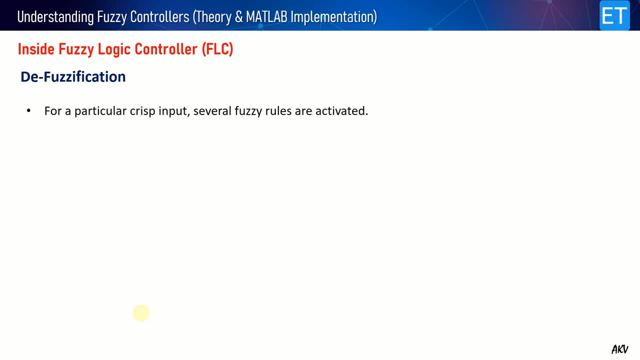 So now let's see what is the defuzzification for a particular crisp input, several fuzzy rules are activated. So according to these activated rules, the output of the inference engines are some aggregated fuzzies sets- Okay, not the crisp values. So from these aggregated fuzzies sets we need the single crisp value so that it can be used. 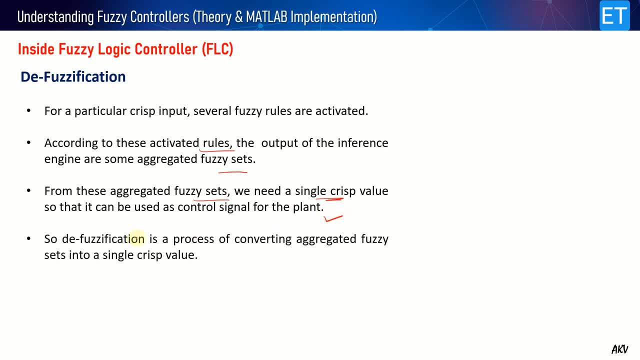 as a control signal for the plant. So defuzzification is actually the process of converting aggregated fuzzies. Aggregated fuzzies sets into the single crisp value. So we have the several methods used for defuzzification, such as center of the gravity weighted average. 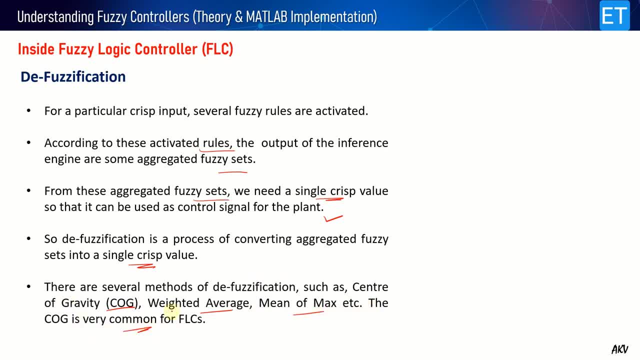 mean of max etc. Where the COG is very common for FLCs. So this is an example of the defuzzification. So here you can see that these two sets are aggregated. So you are getting this total final yellow area as a fuzzy output of the inference engine. 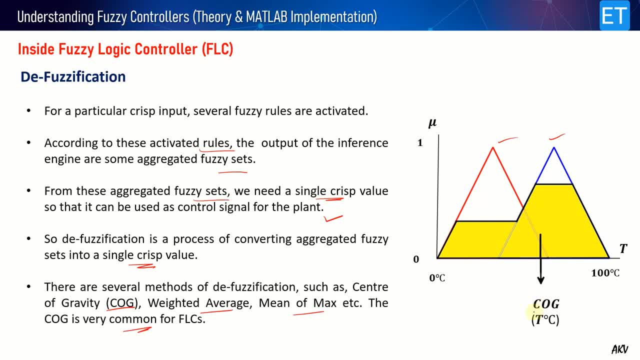 So to convert this into the single crisp value. so we have used the center of the gravity method. So for this overall yellow area we have found this crisp value, some T degree Celsius, as the output. So that is the use of center of gravity. We can use other methods also. 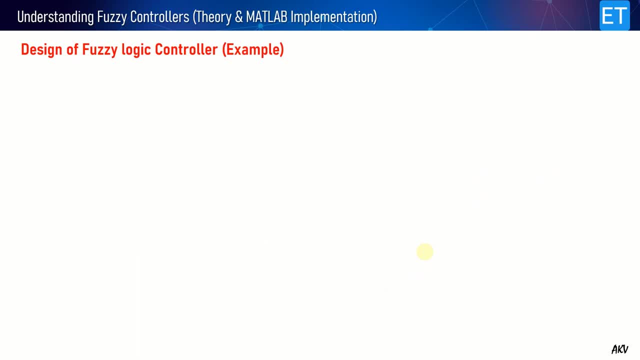 And now let's see the example that how we can design a fuzzy logic controller for certain applications. So here our objective is to design a fuzzy logic controller for the throttle control for a steam turbine. So here inputs are actually the temperature, T and pressure, P of the steam and the output. 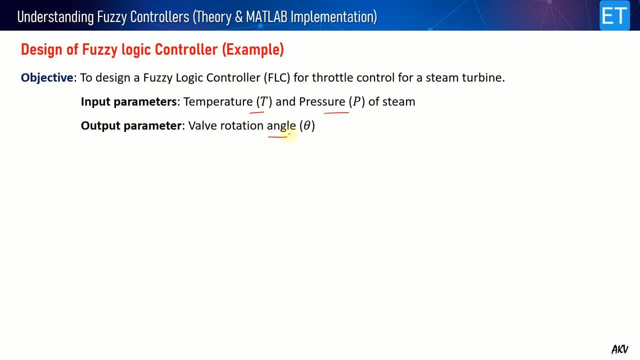 is the rotation of the valve. So that is the rotation angle theta. So this is your controller for FLC inputs- temperature and pressure- and the output valve- rotation angle- theta. So here we are, taking the range of the temperature from 300 degree Celsius to 600 degree Celsius. 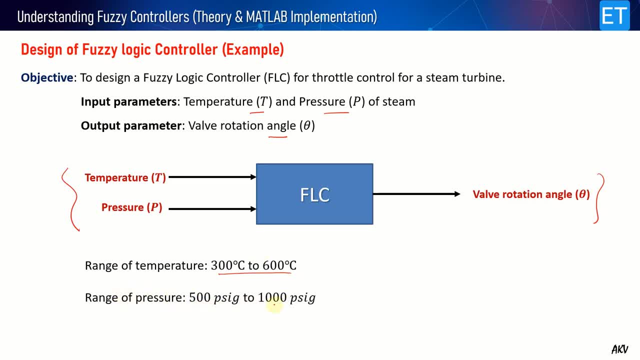 and we are taking range of pressure of steam from 500 to 1000 psig and range of the valve rotation angle from minus 90 to plus 90. So we are assuming that this is a valve at zero degree. it is at the normal position. 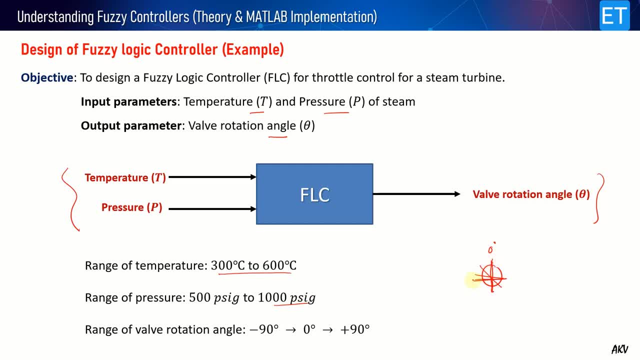 So you can rotate it to the left side till 90 degree, And you can rotate this to the right side to 90 degree. So total rotation is from minus 90 to plus 90, depending on the control action. So now the first step is a fuzzification. 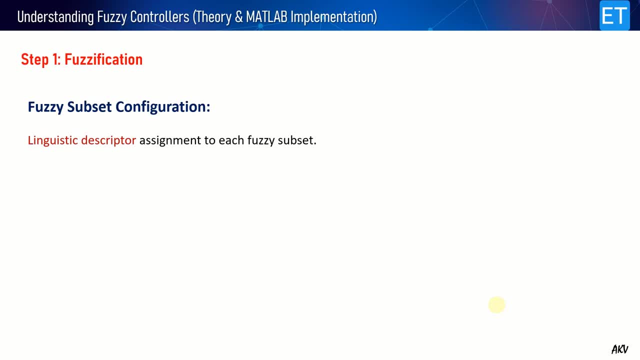 So we have to define the fuzzy subsets. So we are first defining the linguistic descriptor for the each fuzzy subset. We have the two inputs, temperature and the pressure. So we will define the linguistic descriptor for both temperature as well as pressure. So for temperature we have taken the three descriptors: normal, hot and super hot. 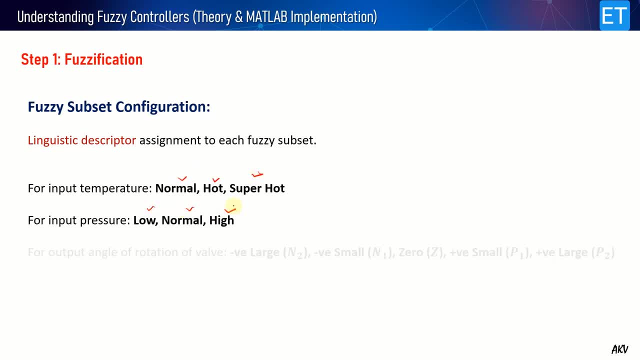 And for pressure, we are taking low, normal and high. And for valve rotation angle, we have taken total five linguistic descriptor zero, that is Z. And then the left side rotation, small rotation, That is negative, small, N1. or negative large, that is N2.. 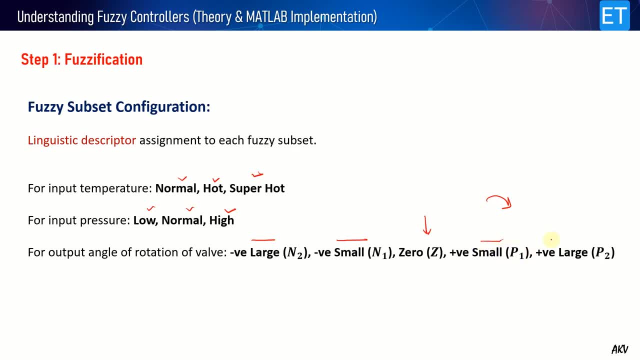 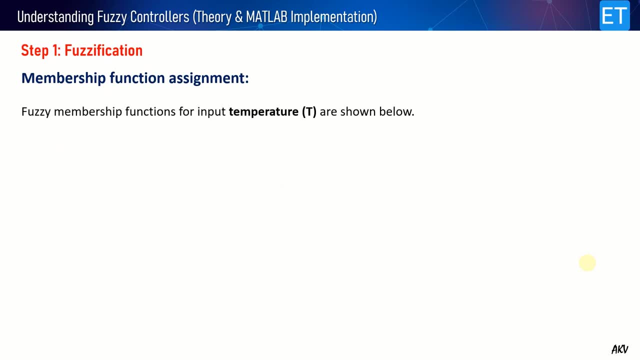 And for right side rotation, the positive small P1 and the positive large P2.. So now let's talk about the membership function assignment, That how we can assign the membership functions for both the inputs. So first we will talk about the temperature. So this is how we have assigned the membership functions. 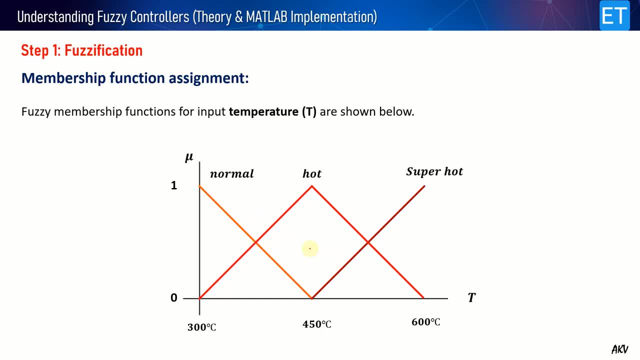 Here we are using the triangular membership function. Here we are using the triangular membership function. Here we are using the triangular membership function. You can use other shapes also. So for three linguistic parameters- normal, hot and super hot- We are assigning these membership functions. 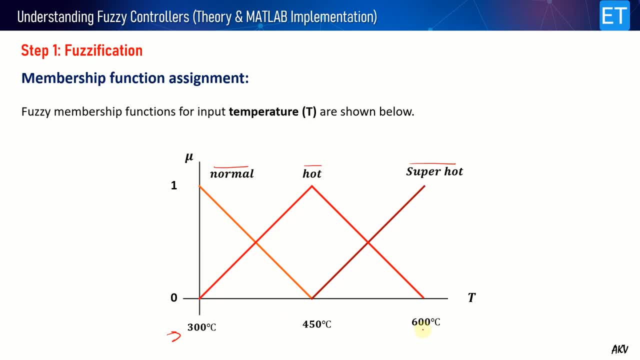 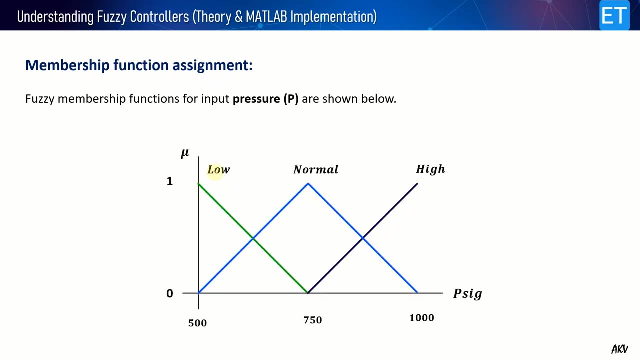 So this is our input range from 300 to 600 degree Celsius And the output is always be from zero to one. That is the degree of the membership, And similarly for pressure. So we have used again the three membership functions for low, normal and high. 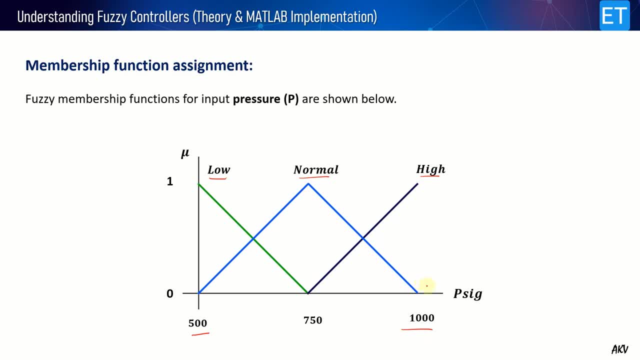 For the range 500 to 1000 PSIG. And now let's talk about the output wall rotation angle, theta. So we have used the five triangular membership functions Z. I mean zero, positive, small, positive, large, negative, small and negative, large. 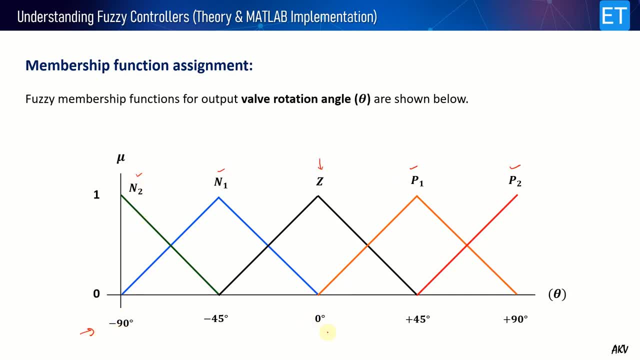 Range we have already decided: Minus 90 to plus 90.. Through minus 45, 0 and plus 45. So zero is the mean projection of the wall. So now let's talk about the fuzzy rules. How to define the fuzzy rules? 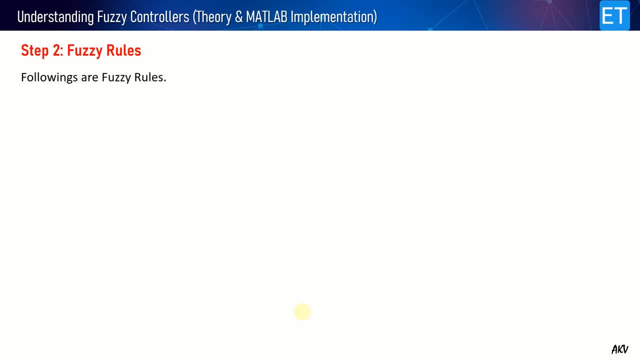 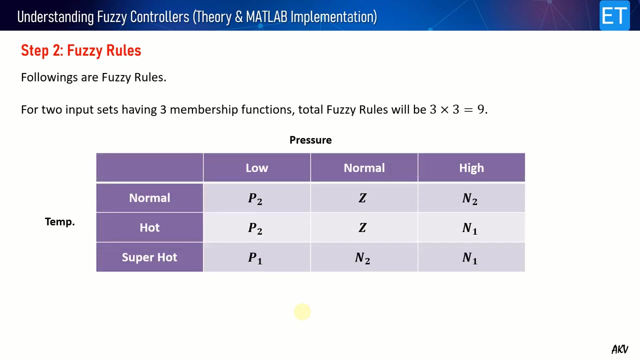 As I said, this is the difficult part and it depends on the experience of the designer. So we have the three membership functions for each input, We have two inputs, So total nine rules will be designed. So this is how we have. So this is how we have thehalcom. 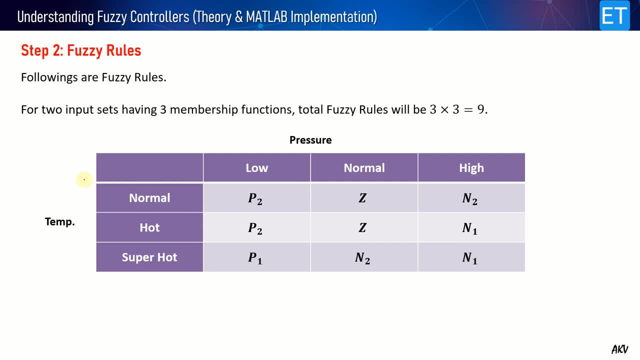 Okay, Okay, arrange all these rules in a tabular form. so here you have the temperature, so normal, hot and super hot, and here you have the pressure: low, normal and high. and here you have given the output action of the wall. I mean if temperature is normal, pressure is low, then your output is p2, I mean the positive large. 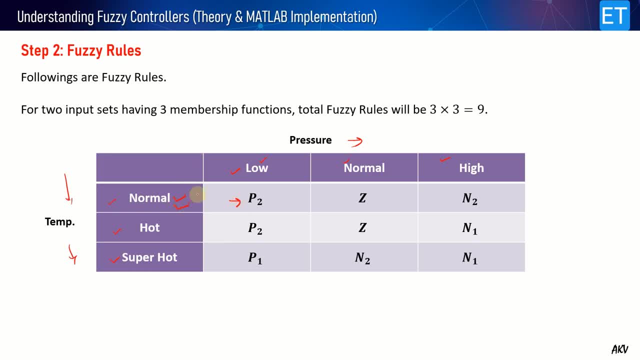 you will open the wall. if your temperature is normal, pressure is also normal, then output action is that do nothing. if temperature is normal, pressure is high, then your action is negative, large I mean you just close the wall like that. similarly, for all combinations you have these output. 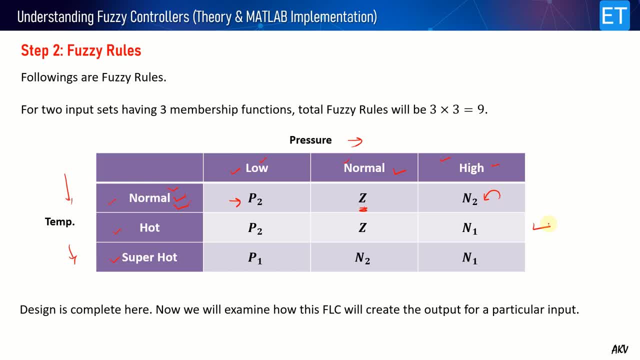 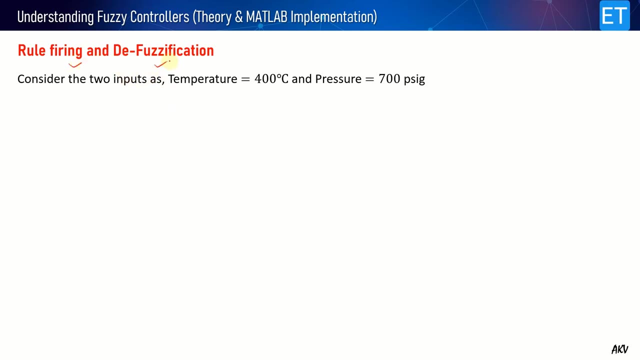 actions. so design is complete at this moment. so now we will examine how this FLC will create the output for a particular crisp input. so for that we can see how the rules are fired and how the defuzzification takes place. so now I am considering one crisp input case where temperature is. 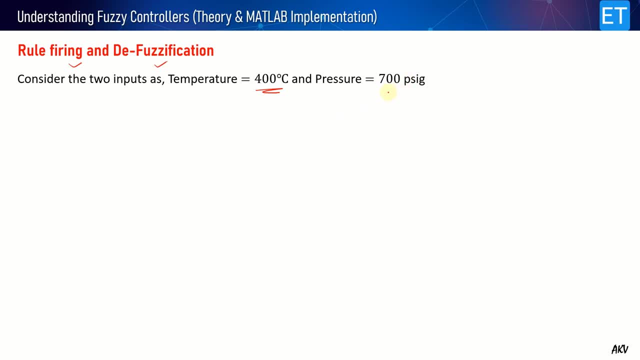 let's say 400 degrees Celsius and the current steam pressure is 700 PSIG. so in this current situation, what will be the corresponding output of this FLC? how much wall it will open in left side or right side? how much angle the wall will rotate. so in this case, what will be the corresponding output of this FLC? how much wall it will open in left side or right side? how much angle the wall will rotate? 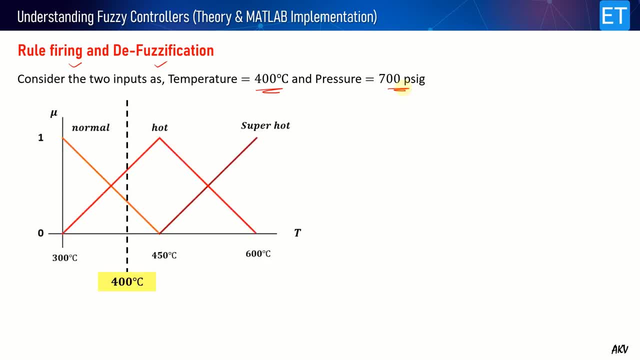 it. let's see so what we have to do. we have to draw the membership functions of temperature and the pressure. okay, so now you draw one vertical line for 400 degree celsius, this one, and for vertical line for pressure, 700 psig. so here you can see that this line is cutting at the 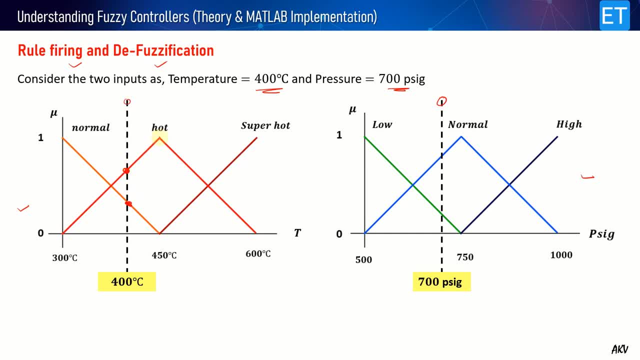 two points. there are two intersection points. it is cutting the hot as well as normal temperature. it is cutting the normal pressure and the low pressure. okay, so we get the four intersection points: hot and normal in the temperature and normal and low in the pressure. okay, this is for. 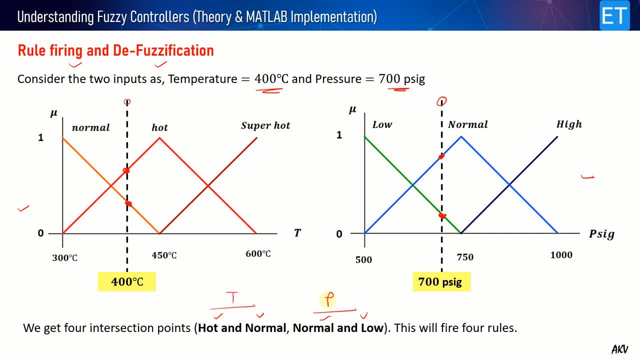 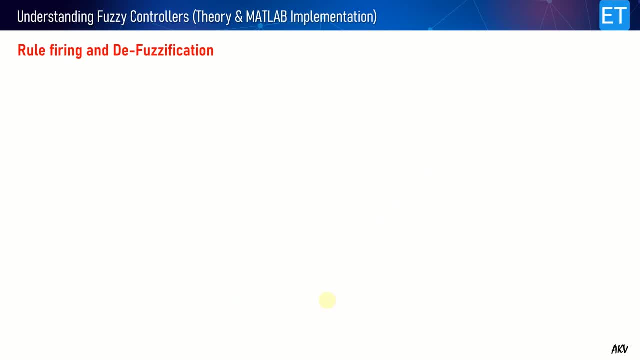 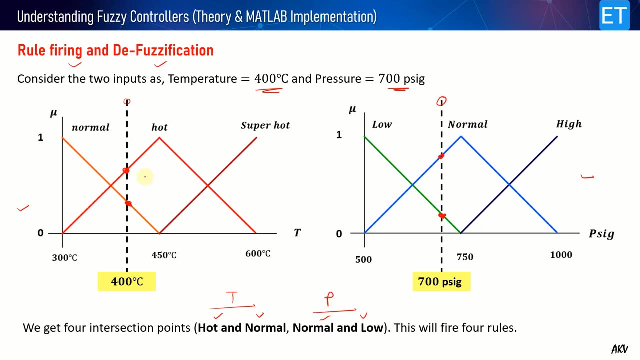 t and these two are for pressure. so because of these four intersection points, total four rules will be fired. so let's see how. so what, we will see. we will actually make the uh, you, the combinations of these four points. i mean, for example, that this is a hot intersection point. 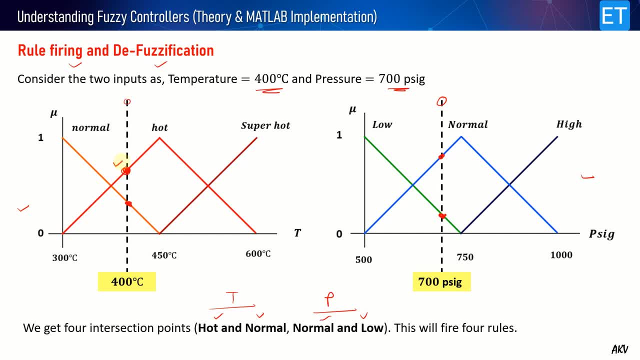 so i will say: if pressure- sorry, if temperature- is hot and then pressure is normal, what is the output action? if temperature is hot, pressure is low, what is the output action? similarly, if temperature is normal, pressure is normal, then what is the output action? if temperature is normal, pressure is low, then what is the output action? so that we will search in that. 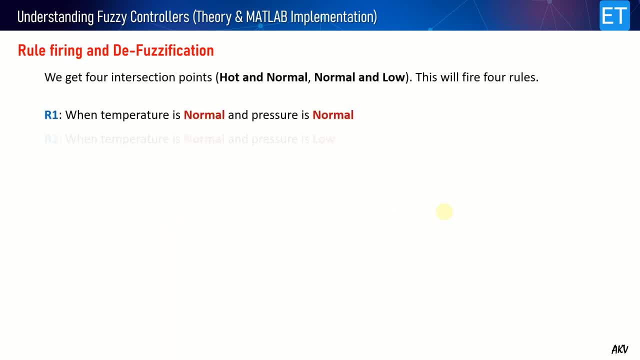 rule table. so let's see how. so i have uh written all these four rules, that when temperature is normal and pressure is normal, when temperature is normal, pressure is low, temperature is hot, pressure is normal and temperature is hot and then pressure is low. so what will happen? what will be the output? 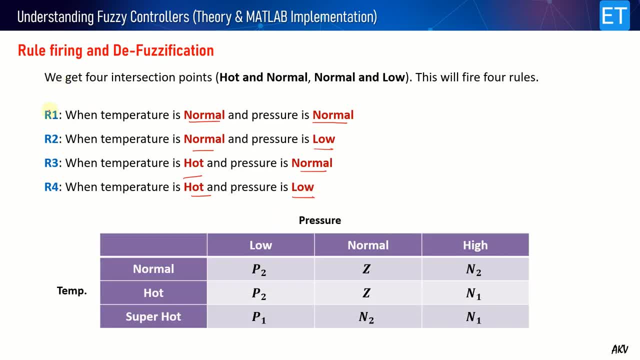 action. so just recall that table. so we'll take the rule one: when temperature is normal and pressure is also normal, then obviously the rule fad is this: that means output, is that do nothing with the wall p. so for r2, when temperature is normal and pressure is low, obviously p2 is fired. 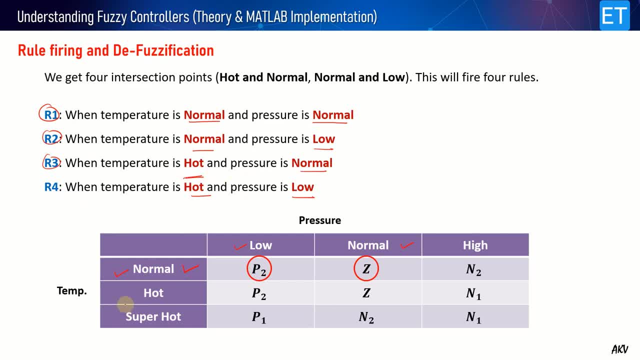 rule three: when temperature is hot- this one- and pressure is goes down and you essentially have the non- approximated ç, whose output z does not match the pressure normal, then this is a rule. rule 4: when temperature is hot and pressure is low, then this is a rule p2. 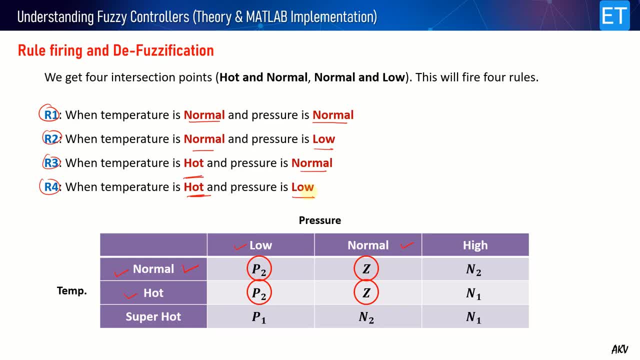 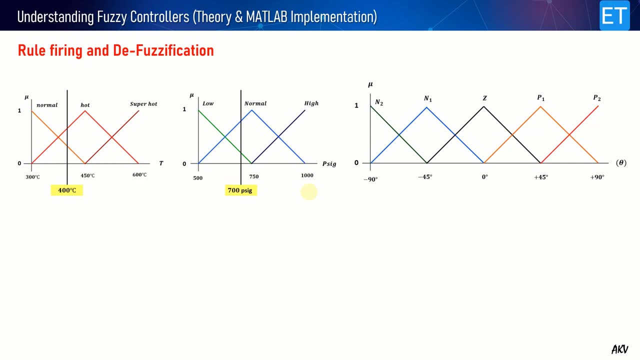 so we have these four rules that will be fired for this combination of the temperature and pressure input. so let's see how we'll get the output. so now draw all the membership functions side by side like this: you can draw this on a graph paper, also with a certain scales. so we'll first 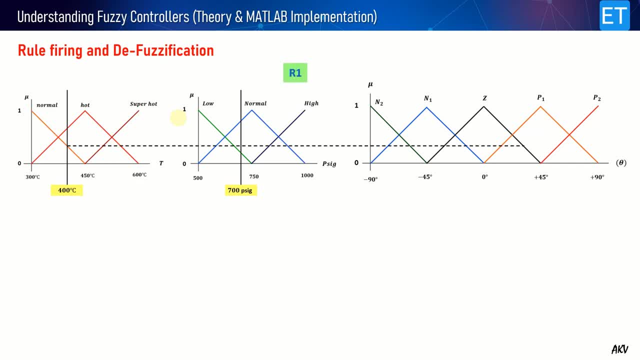 show the rule one. rule one: okay. so this is the horizontal line which is showing that the temperature is normal. when temperature is normal and pressure is normal, what is the output? output was a z. okay, so since here we are using the end operation, so we are using actually the min operation, so we will highlight the minimum one. 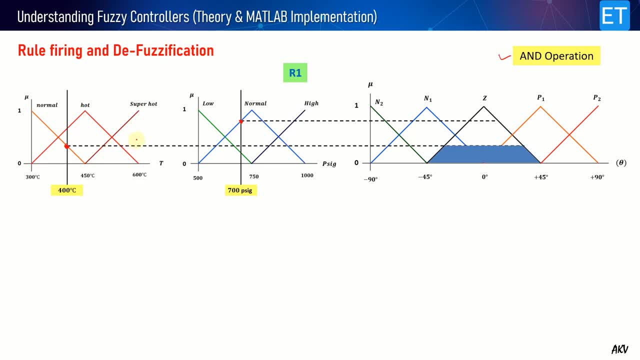 so, since output action is z, so we will take the minimum value and we will highlight this area under the z membership function. so this is the rule one: activation is complete. now come to the rule two. okay, in rule two, when temperature is normal and then pressure is low, 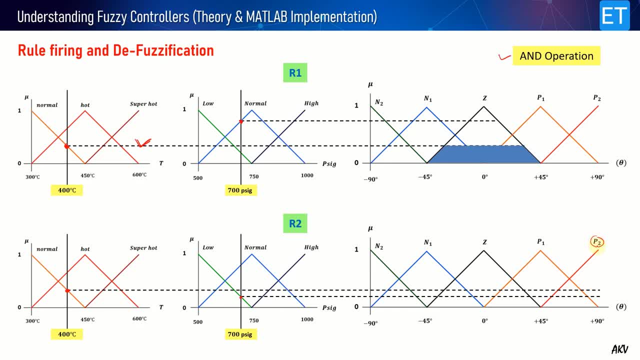 then output is p2 and since because it is a end operation, so we will highlight the minimum area, okay, under the p2. so this is, the p2 rule is activated. so now two more are remaining: rule three and four. so let's come to the rule three. 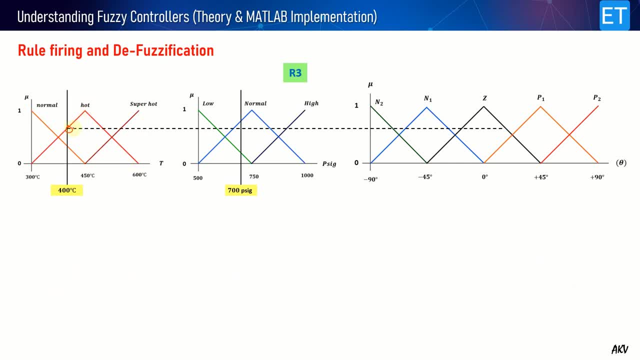 when temperature is hot- okay, that is a hot intersection point- and the pressure is normal, your output is z. from that table, which we have already discussed, and because of the end operation, we'll highlight the minimum area under the z right. so rule three is complete. similarly rule four, uh. where temperature is hot and the pressure is low, pressure is low, the output. 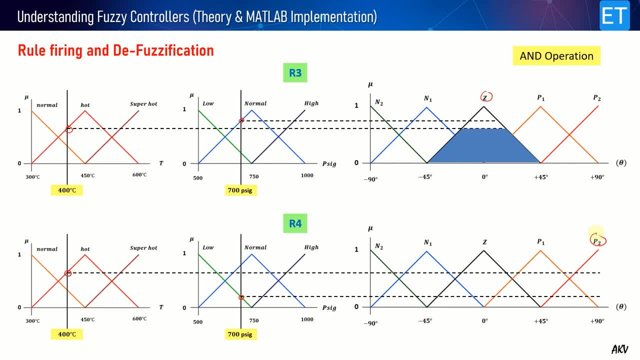 is p2 from that table and because of the end operation, we will highlight the minimum area right. so we have seen the activation of all the four rules here. this exercise. if you want to do the manually, you can do this on the graph paper. okay, so you can get the actual values of these uh points. 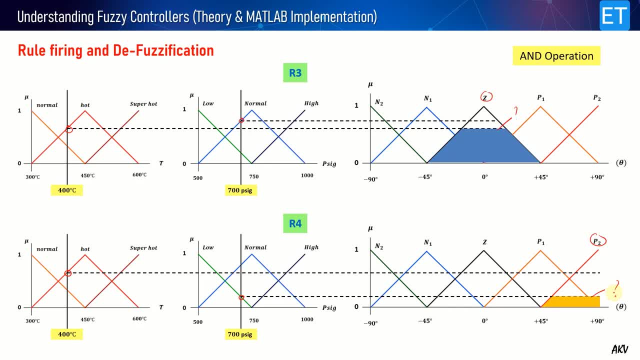 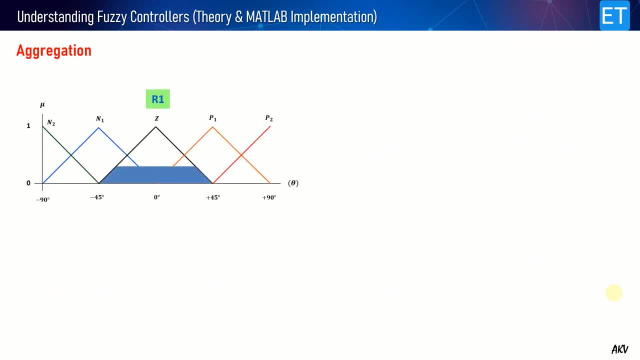 all the numerical values of these heights. so now we'll do the aggregation. so first let's see the area under the z. in two rules, r1 and r3, we got the z output okay. in one we are getting this much height, in r3 we are getting this much height. so which one we have to take here for aggregation? we actually 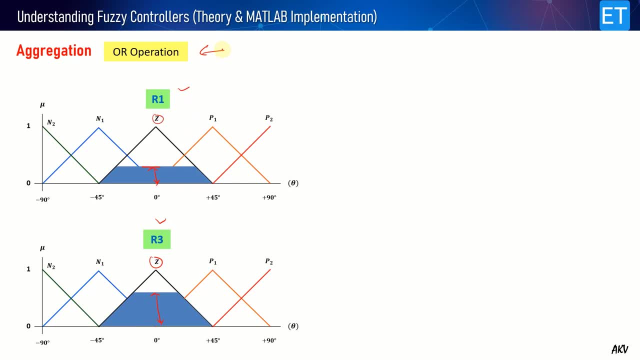 go for generally our operation. so our operation means the max operation. so we will take as a max area, maximum height, i mean this one. so let's say this height is mu 1. so that is my aggregation of the area under the z. similarly, in the remaining two rules- i mean r2 and r4- we are getting the area. 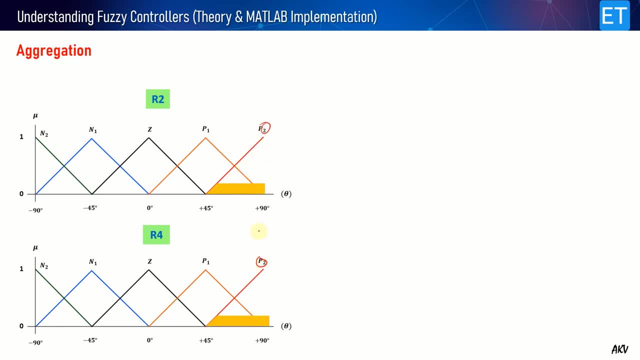 under the p2. okay. so again, we will apply the or operation and we will aggregate and we get the single outcome as this: which one is the larger? but if you draw this on the graph paper, you will see that in this particular case both are having the same result. so we are getting the same result. so 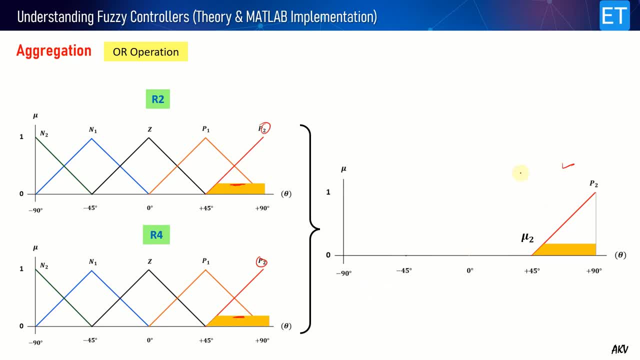 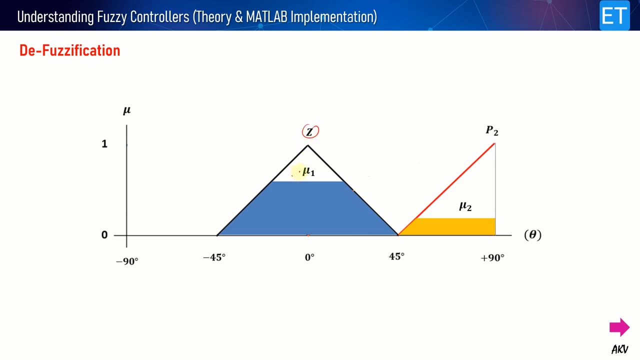 both are having the same magnitude, same height. okay, so we are getting this. let's say, this height is mu 2. so now you just, uh, put all the aggregated areas together for the diffusification. so under the z, we are getting this mu 1 height. under the p2, we are getting this mu 2 height. so just consider. 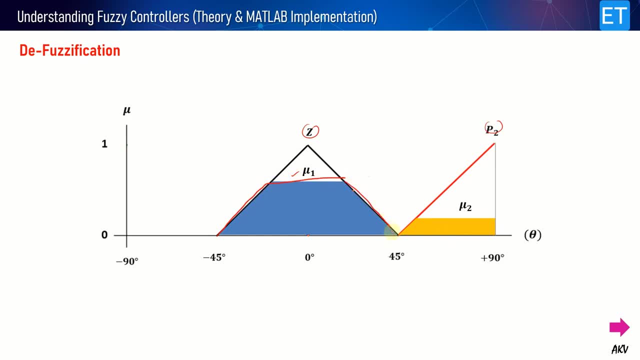 this as a single combined area and now you have to do the defuzzification to get a single crisp output. okay, so this is, these are actually the fuzzy values, and we have to get the output using the defuzzification. so here i'm applying the center of the gravity. so with help of the center of gravity, i find this as cog. so on x-axis i mean. 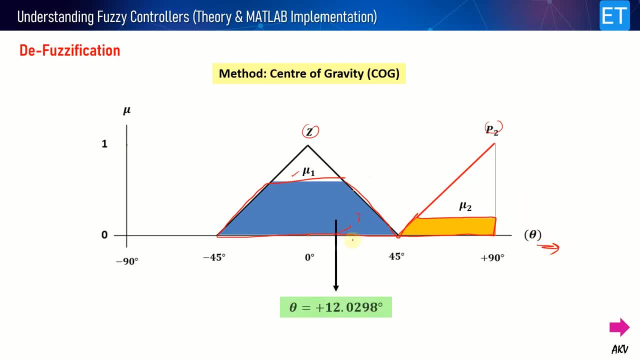 on angle axis. let's see how much angle is this? this is a plus 12.0298. so it means uh for uh, 700 psi g pressure and 400 degrees celsius of the steam temperature this flc will create or it will open the wall: uh 12 degree in clockwise direction. i mean this is a z point, zero point, and it will be. 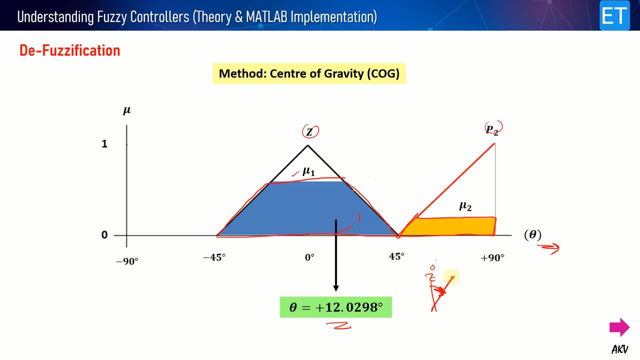 slightly open the you uh valve to let the steam uh pass more, more steam. so that is 12.0298 degree. okay, so this is how the flc gives output. so for any input combination you can try within the range of temperature and pressure. you can try any combination and you will get the output. so this is the complete process. i. 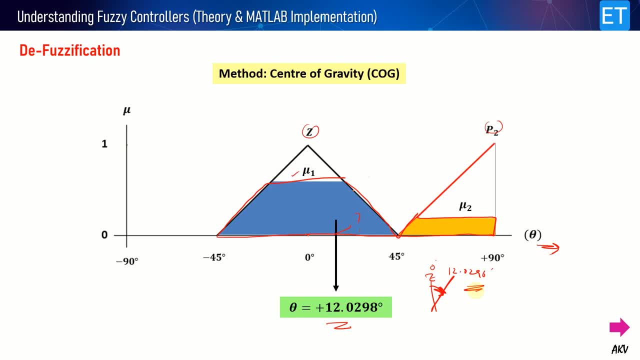 hope you have understood this process. if you want to do this manually, you can do it manually. do this on the graph paper. you follow all the steps on the graph paper. with a certain scales you will get this 12.0298 degree. okay, manually also. so now the 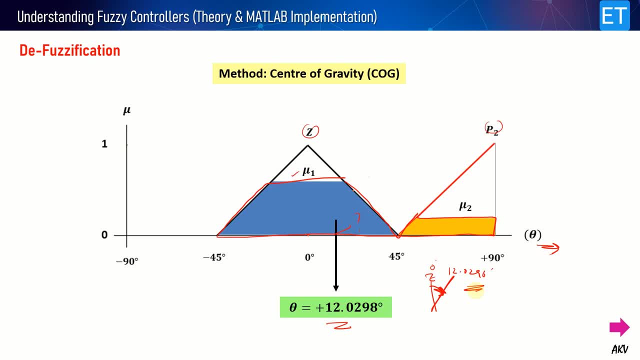 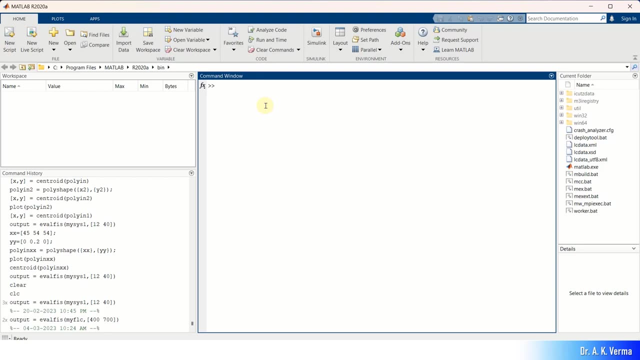 time to implement this in matlab. so here i will show you that, how you can implement this flc in matlab. so let me jump to the matlab and this is my matlab. so to implement this flc in matlab, if you want to implement this flc, you needframe기 and you need televlet. 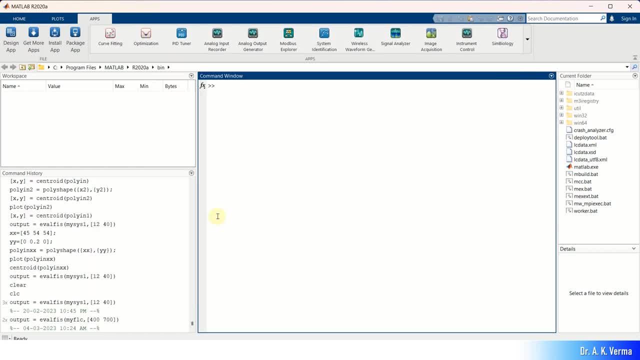 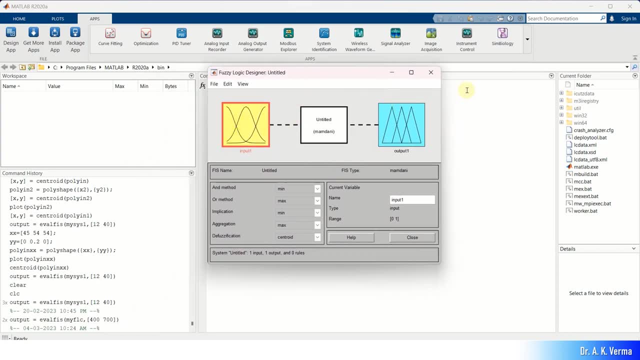 environment to implement this. it's the same as the what you upfront saw, and then the system mc on linear, between static and private, and you will automatically getson in malware platform which is called ftflenuxyid. if you have an, ourselves wasn't using this framework. 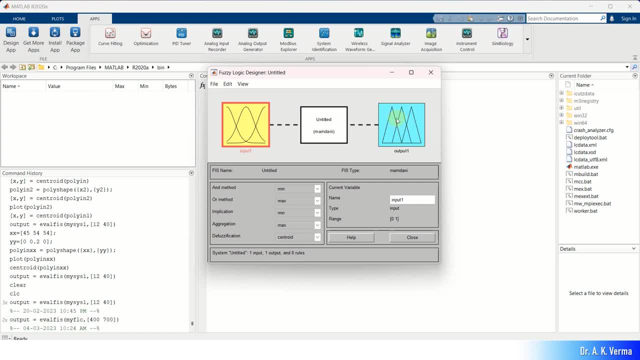 And so these are the input membership functions and these are the output membership functions And in between, this is a rule-based block. So since our system has the two inputs, so we have to add one more input. So go to the add it. add variable. add variable input. 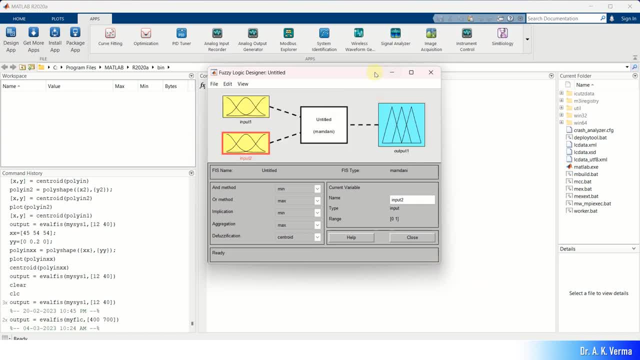 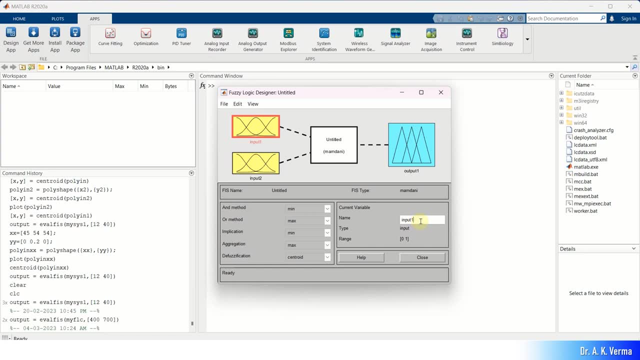 So now you have the two inputs. You can see two inputs, So now just go to the input one And you can change its name. Default is input one, So you go to change the name. Let's say, let me write the temperature. 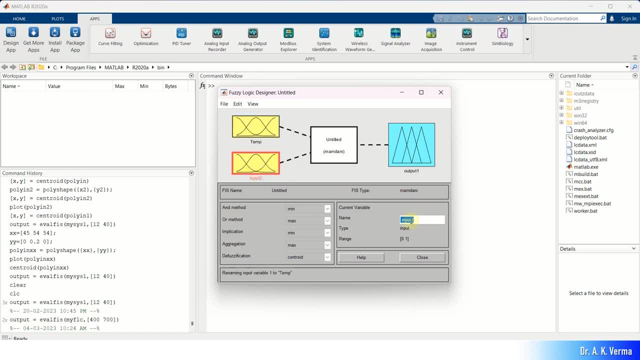 And for second, let me write the pressure Pressure, okay, Temperature and pressure. And similarly for output, you can change the name. Let's say theta. Theta is my output, Okay. so now let me define the membership functions. So just double click this temp temperature block. 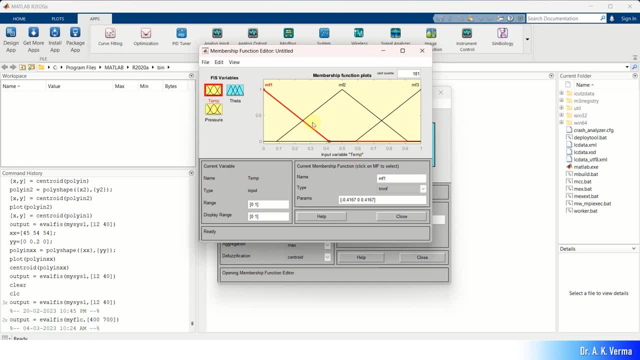 So here, by default you have membership functions. Better to remove all these membership functions, So go to the add it. remove all MFs, Okay, so you have a blank window. Now go to the add it again. add MF. Okay, so from here, MF. 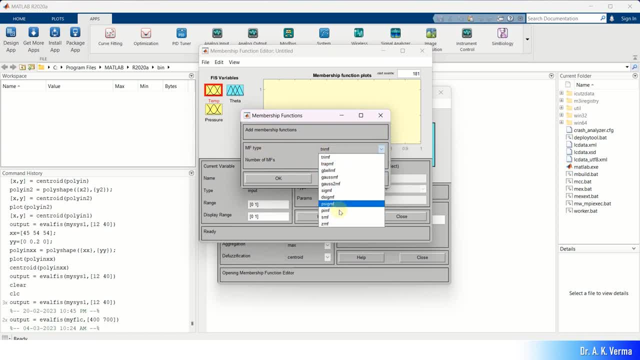 Type. you can choose any membership function type, like Gaussian Bell type, trapezoidal, etc. So here I am using the triangular, So that is by default triangular membership function and the number of membership functions. So, as we have seen that we have chosen the three membership functions, 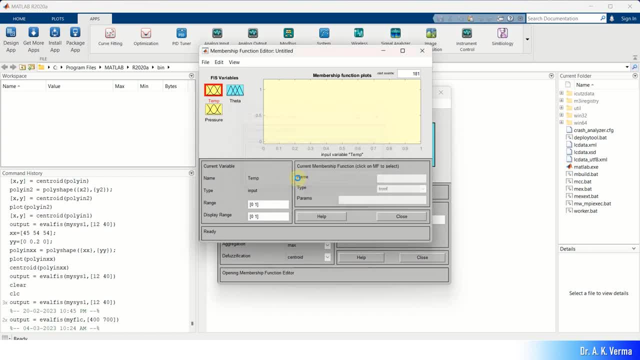 for temperature and pressure input. So just press okay, You get these three membership functions. So their default name is MF1,, MF2, and MF3.. You can change their name from here. So this is actually. we are working for the temperature. 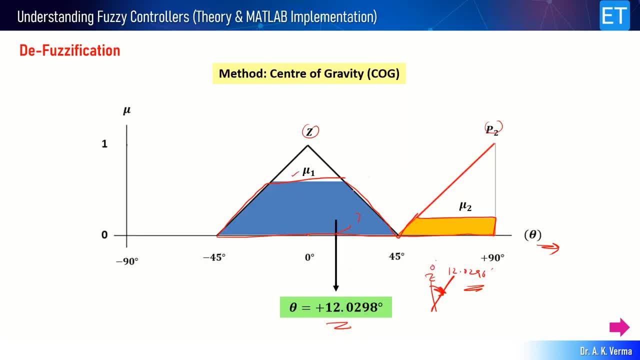 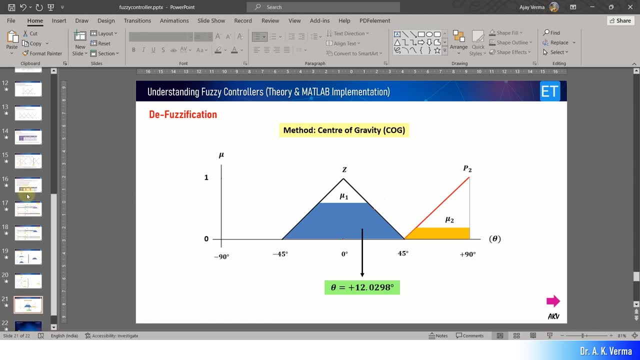 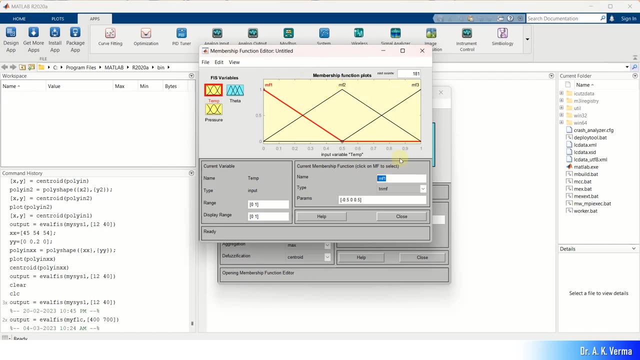 So for temperature we have taken the name. Let's see which name. For temperature we have three linguistic variables: normal, hot and super hot. So the first one is normal And then second one is hot And third one is the super hot. 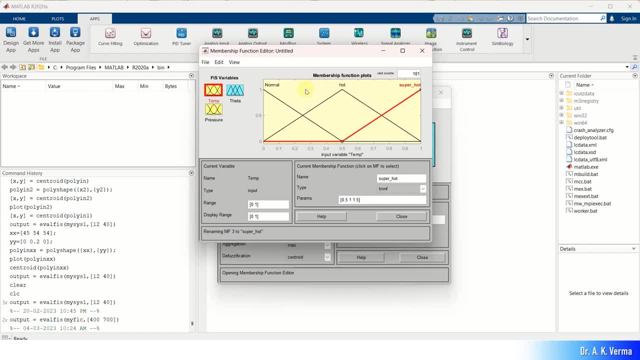 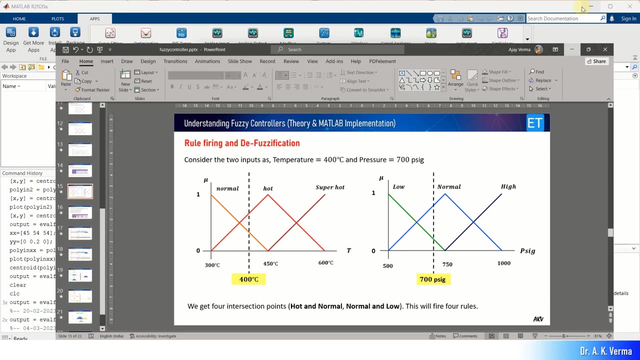 Okay, so this is how you can assign these linguistic parameters. And now see the range. Range default on x-axis is from 0 to 1.. But our range was from 300 to 600 degrees Celsius. So here we are. So here we are. 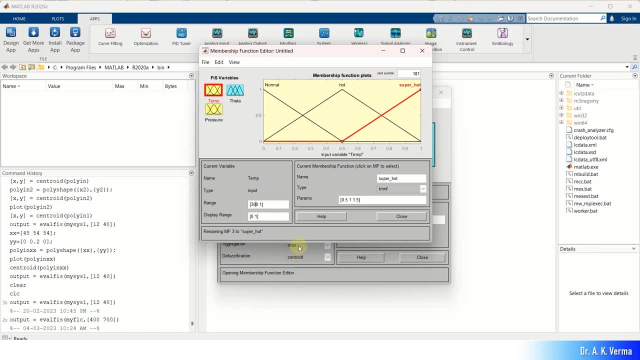 And then second one is hot, And third one is the super hot, And then second one is super hot, And then third one is the super hot, And then third one is the super hot, And here we will give this range 300 to 600. 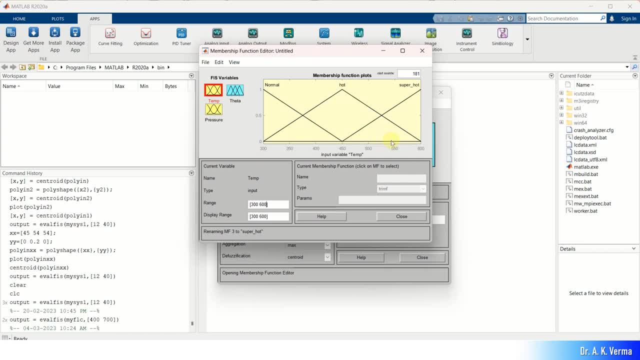 You just press enter So your range is changed from 300 to 600, right? Similarly, I will go to the pressure and then add it. Remove all the MFs. Add it, Add MFs. Okay, So three membership functions are added. 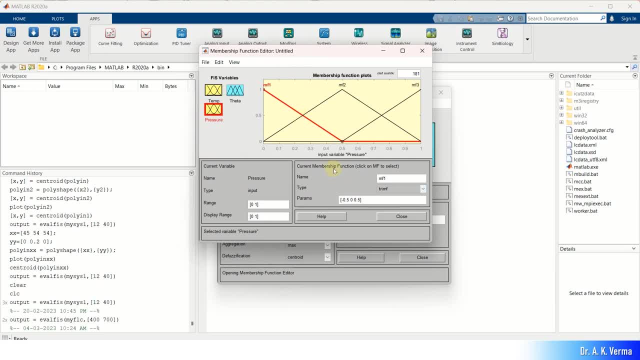 Now I will change their name instead of MF1.. My linguistic assignment is low, normal and high, So this is the low And second one is the normal And third one is high. Third one is the high. Okay, And change the range. 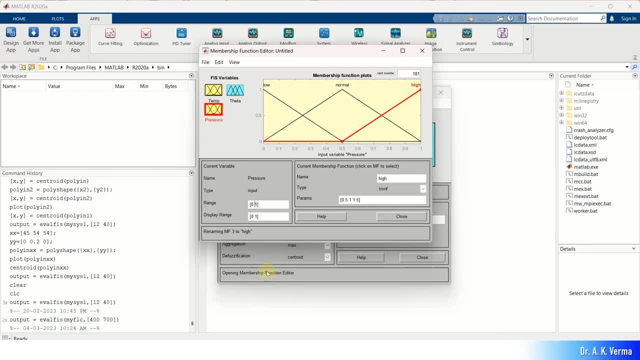 Range is from 500 to 1,000 PSIG. So 500. To 1,000.. Okay, Press the enter So your range is changed And I'll come to the output theta. Again, go to the add it. 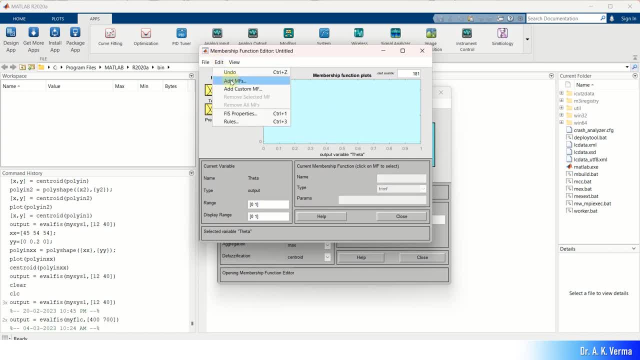 Remove all MFs. Add it. Add MFs And instead of three, choose five, Because we have defined five membership functions. So these are five default membership functions. Share: change their name. The first one is the N2, negative large. 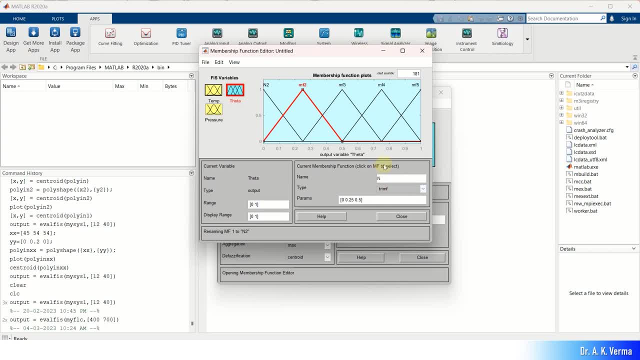 Second one was the N1, negative, small. The middle one is the zero, That is the Z, This one is the P1, positive, small And this one is the P2. That is large, positive, And then change the range. 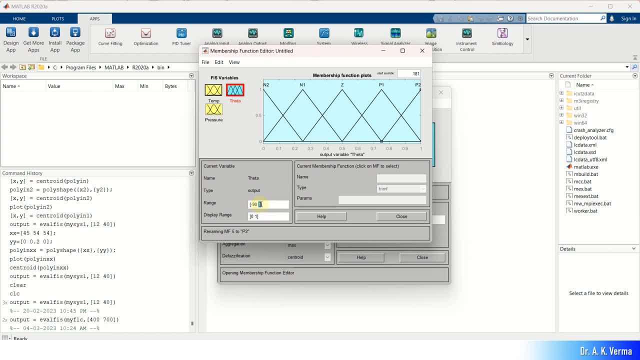 That is from minus 90 to plus 90.. Okay, Okay, So range is changed. You can see from minus 90 to plus 90.. So this is how all the membership functions are defined. Now close it And then go to this middle block. 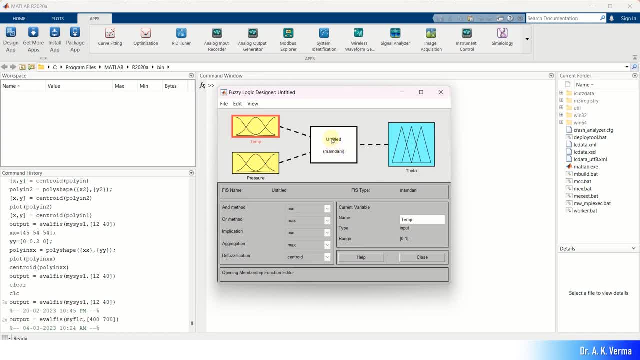 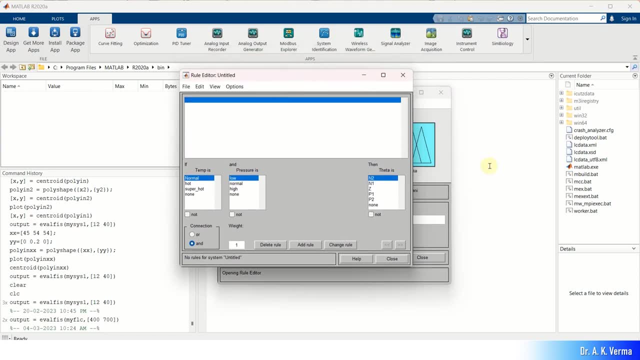 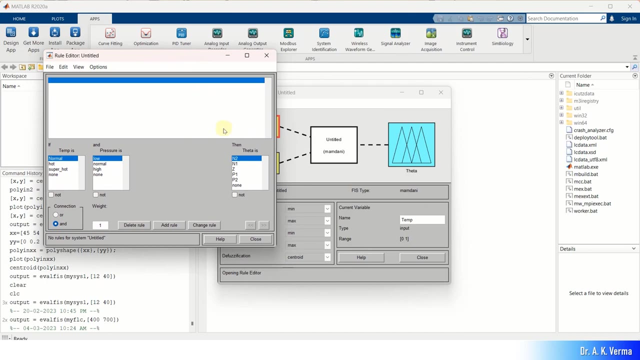 That is your rule actually. So go to the rule fuzzy rules, Double click it And here you will get This GUI where you can add all the nine rules. Okay, So to add the nine rules, you need that table. 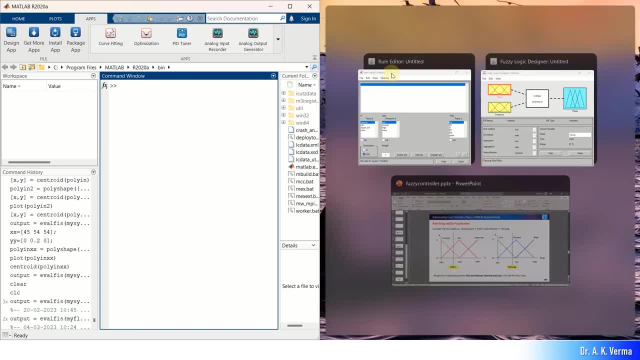 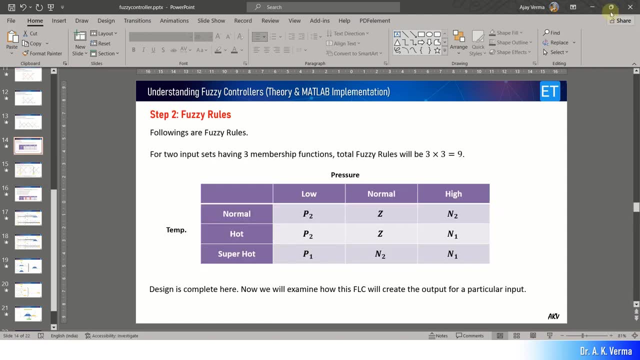 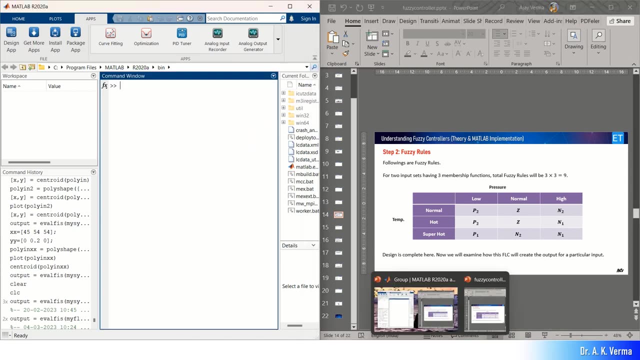 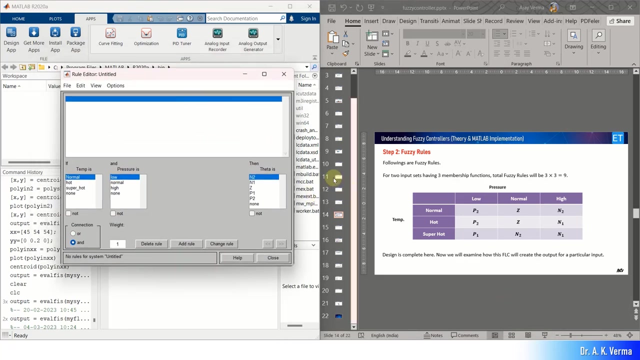 So I will recall that table. Where is that This one? Okay, So this is my table, Okay, Okay, So now I will define all the nine rules. So I will take the first combination when temperature is normal. You see both the list here. 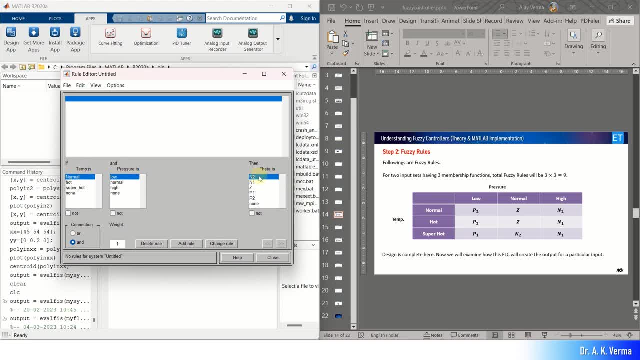 This is first for temperature, Second is for pressure And third one is for theta. So when temperature is normal, you just select normal and pressure is low, Right? So what is your output? Your output is P2.. You just select P2.. 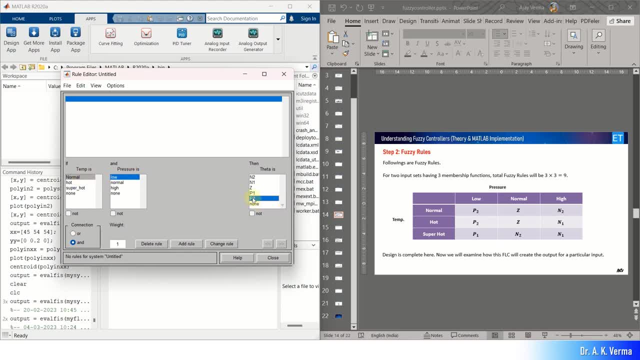 So temperature is normal, Pressure is low And then output theta is P2.. So you just add. So the first rule is added. Now go to the second rule, Sorry. Second rule: Where temperature is normal, Pressure is normal, Then output is Z. 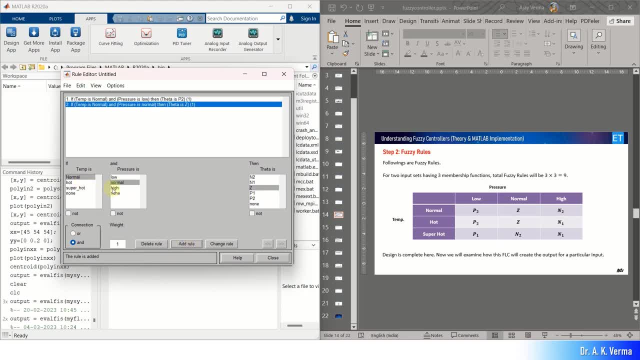 Add rule: When temperature is normal, pressure is high And then output is N2.. Add rule. So the first row is added. Now the second row: Come to the second row. When temperature is hot, Pressure is low, Your output is P2.. 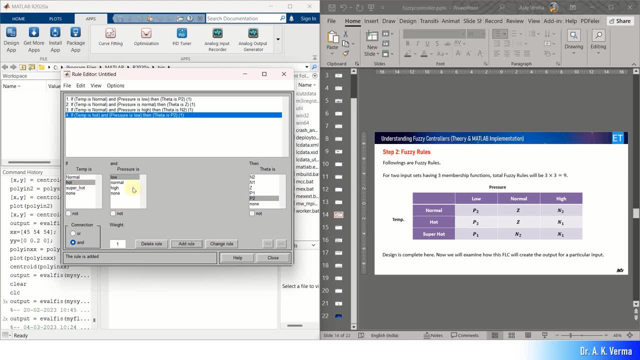 Add rule. Temperature is hot, Pressure is normal, Your output is Z. Your temperature is hot, Pressure is high, Then output is N1.. Add rule. So second row is added. Now come to the third row. Your temperature is super hot. 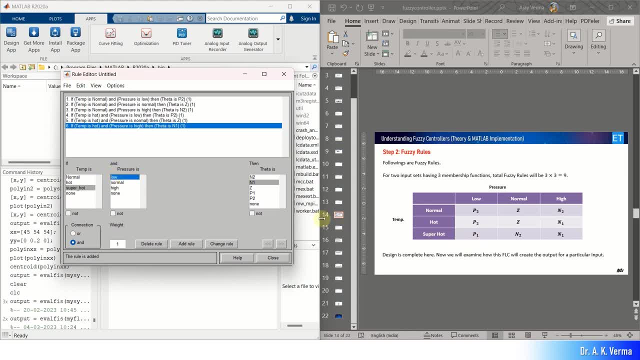 And pressure is low. low, your action output. action is p1, add rule. and then temperature is super hot, pressure is normal. your output is n2. your temperature is super hot, pressure is high, then output is n1. add rules: okay, so all the nine rules are added. i mean this table is completely added here, all one, two, three, 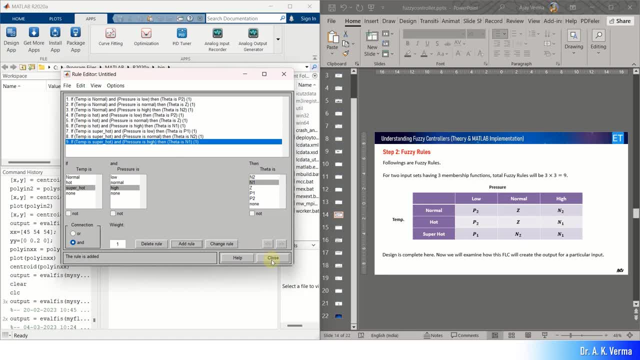 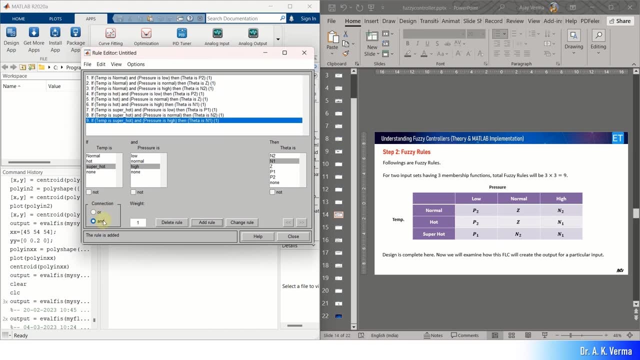 four, five, six, seven, eight, nine, nine rules okay, so you just close it. uh. let's see other things also, like: uh, connection, connection is the end okay. so in the theoretical part also we have used the end operation. i mean minimum will be choose will be chosen during the rule firing, so you can. 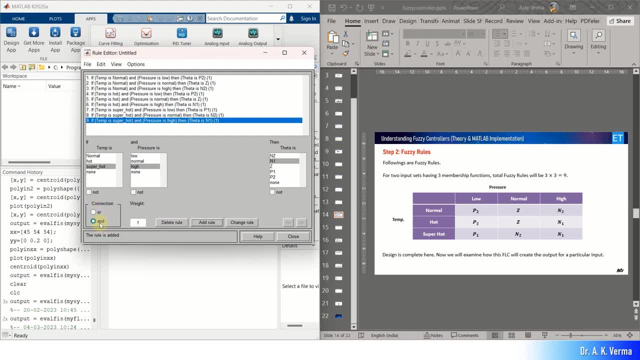 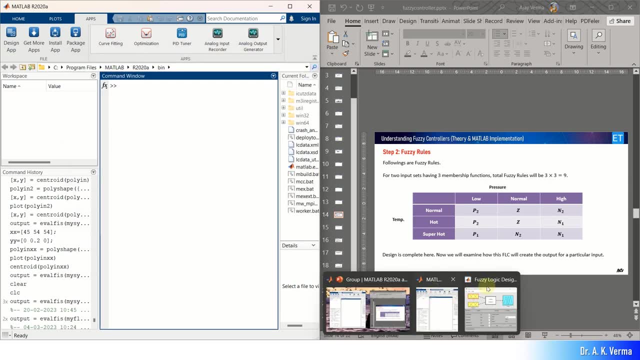 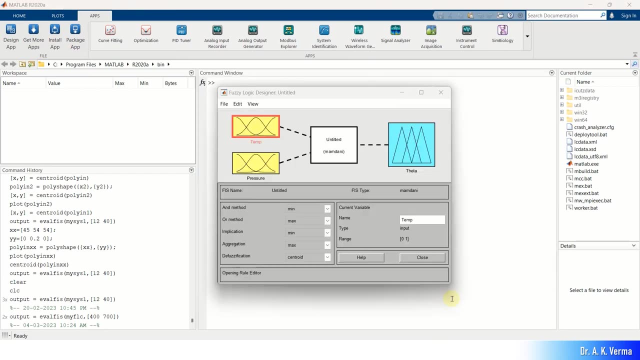 you can have the options of or also, but we are taking the end operation here, so don't change anything else, just close it. so this model is complete. this fuzzy model is complete. so this fuzzy model is complete. okay, and see, uh, the end method is the min method here. 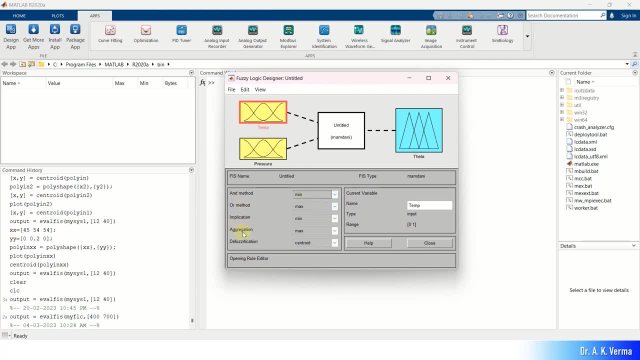 or more, or method is the max method and the aggregation of those fuzzy set is the max and the defuzzification is the centroid. you can choose other also centroid, bisector, max of mean, of max, like that. so we are taking centroid. so now what you have to do. 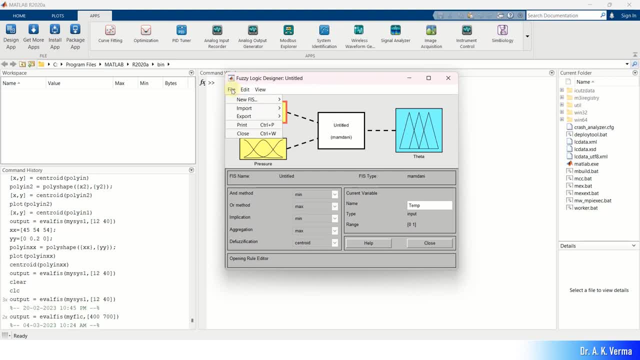 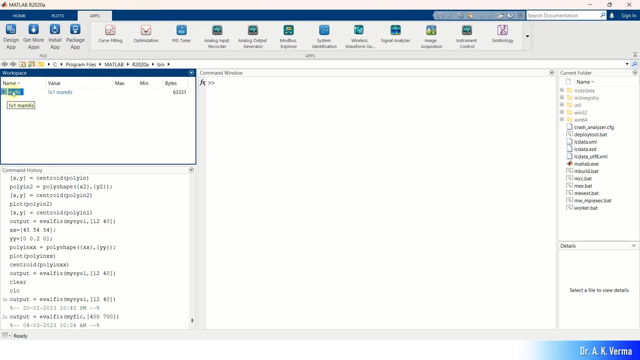 after this we are going to try to set it in to the file. so now you can see consumption snag lcd. okay, all right, go to theew. holy, and there are some checks, but i'm going to say excluding gdp, uh and uh, all right, it's being created. 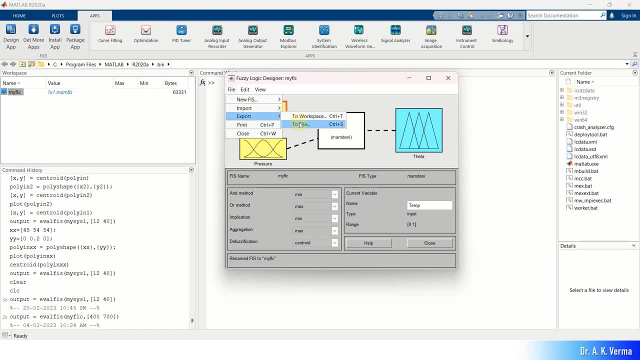 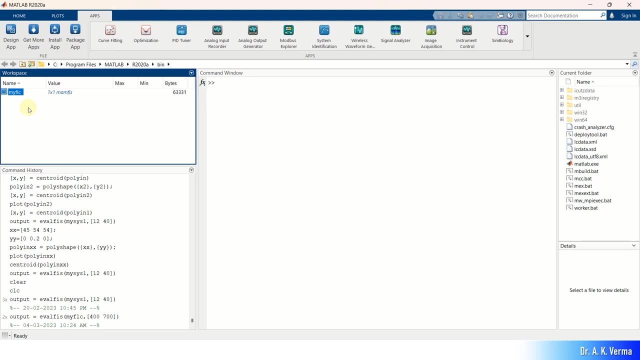 them. You have seen this option to the file, So you can generate this file and you can Utilize this file at some other computers also, right? So just minimize it. even you can close it. So this is. FLC is now made and it is active in the workspace right now. So now let me.